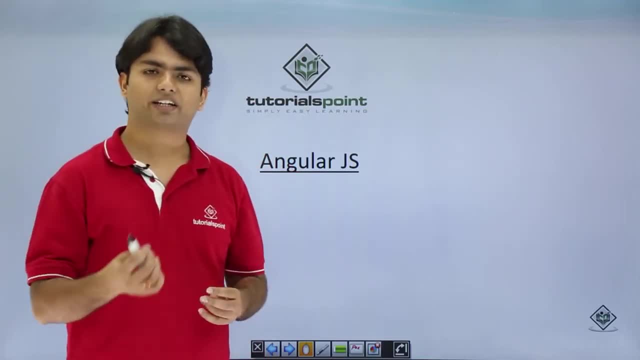 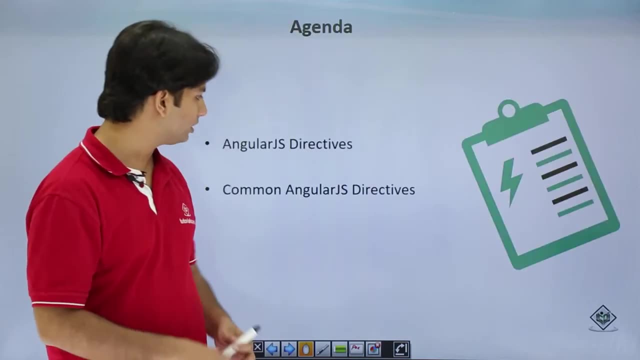 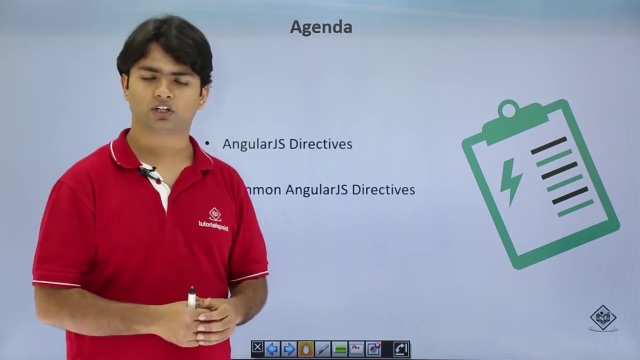 Now in this video we'll cover what directives are all about. Like in the previous example, we have seen the ng-app directive for writing a basic AngularJS application. Here we'll see some more directives- what a directive is all about- and some commonly used AngularJS. 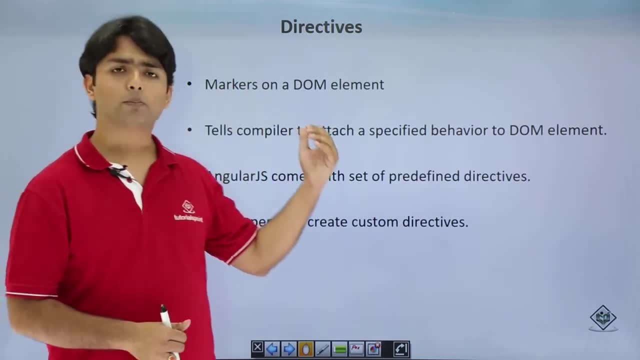 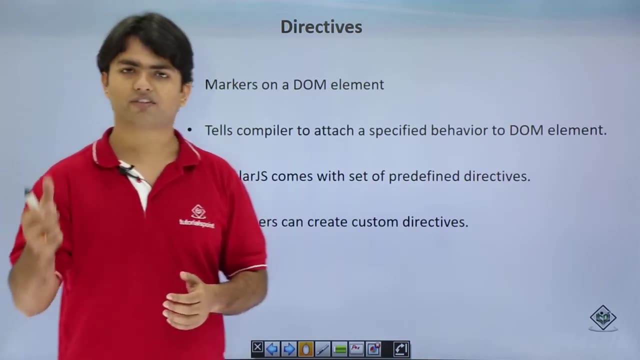 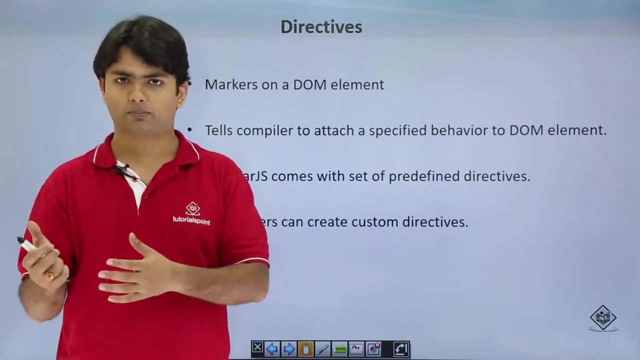 directives. So let's see, Basically, when I talk about a directive, directive is like a marker in the document: object, model Means. whenever you put a directive, it will actually tell a compiler that what particular action needs to take place, right here, For example. 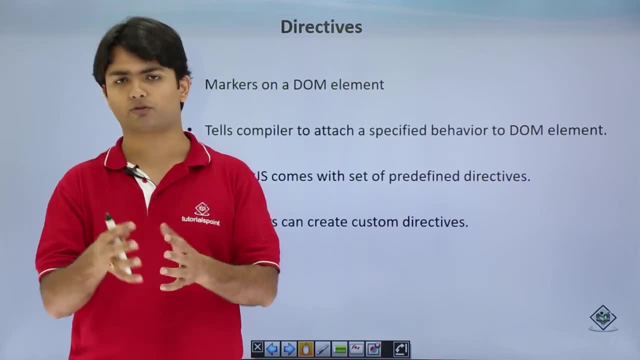 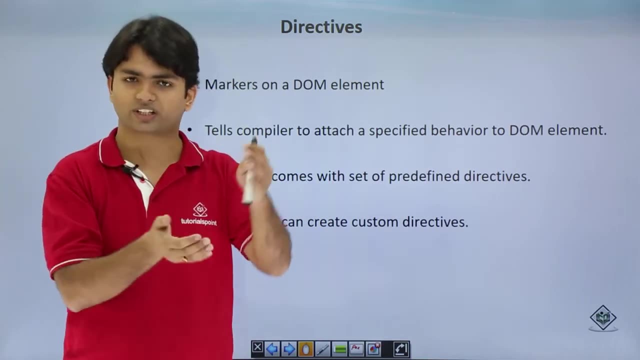 if we have multiple controllers- since here we'll use model view controller architecture- suppose we have created a number of controllers and we want to set a particular controller on a section of a page, So we will have to use a directive for doing the same thing, and 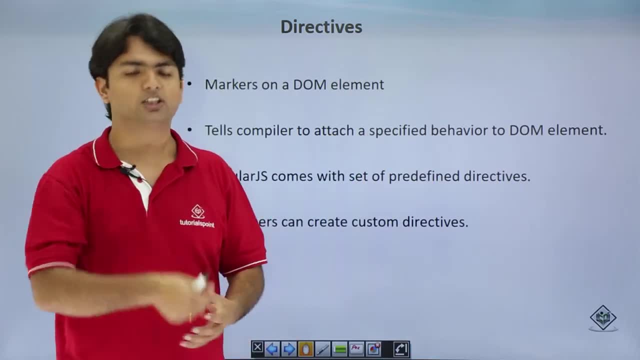 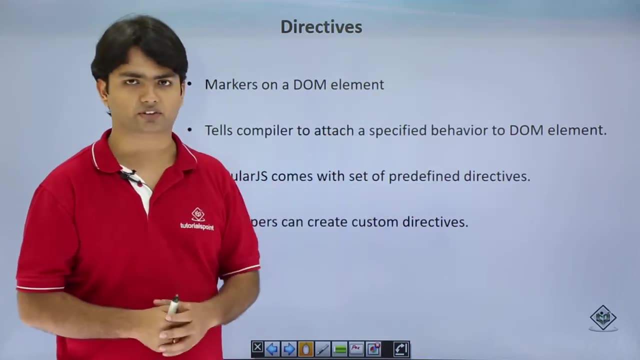 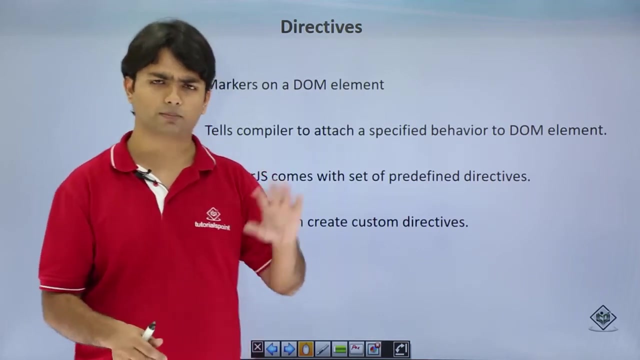 it will definitely tell a compiler that, okay, we are using this particular controller. So these are nothing but some predefined sets of directive which we will see in our next screen. Along with that, we can also create the custom directives, But in this video we'll just focus on the predefined. 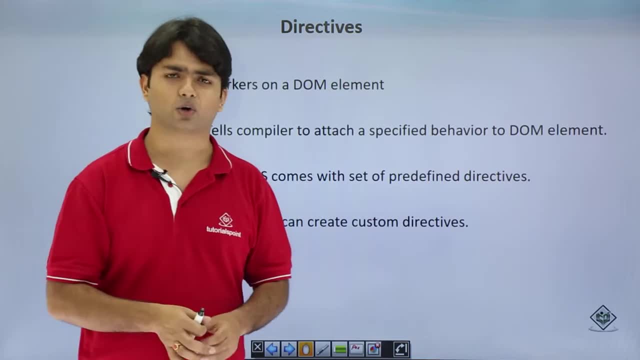 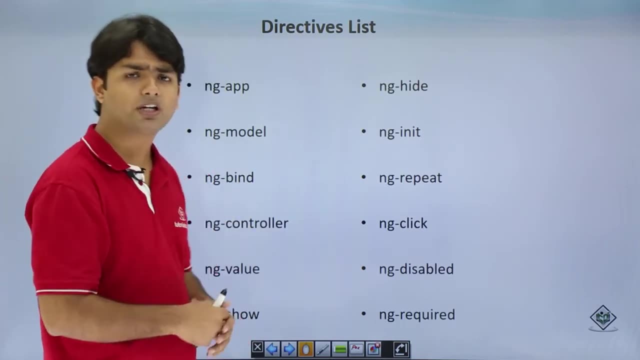 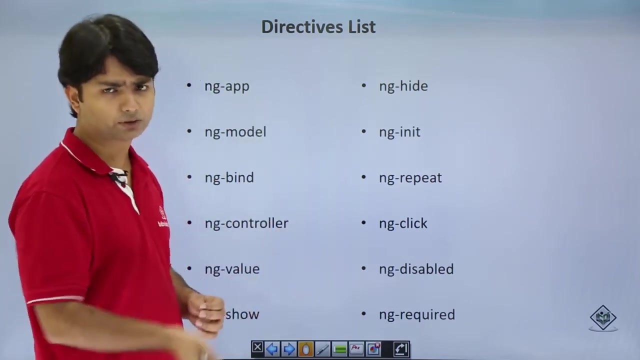 directives which we are getting from AngularJS and we'll see how to create the custom directives later. Now here is the quick list of the commonly used directives As here. first you can see ng-app, Which we use for starting the AngularJS application, as we saw in the previous example. Now ng-model. 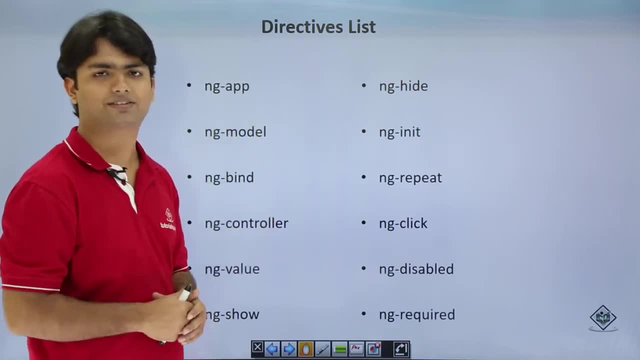 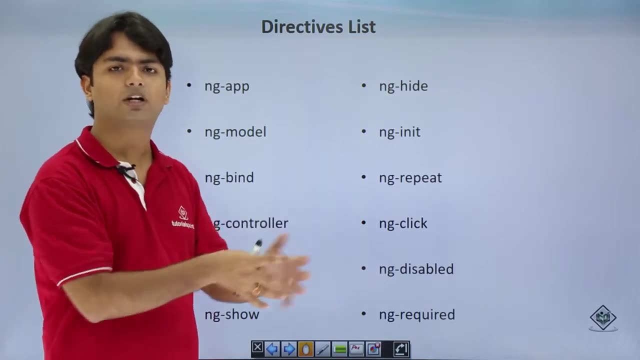 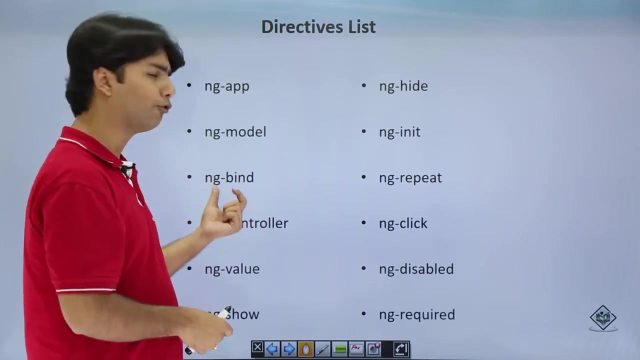 and ng-bind. Basically, both of these directives are used to bind the value, But if you want to bind the value with any HTML control, you will go for ng-model, While if you want to do the same for the tag, you can go for ng-bind. So, for a control, ng-model and for the tags. 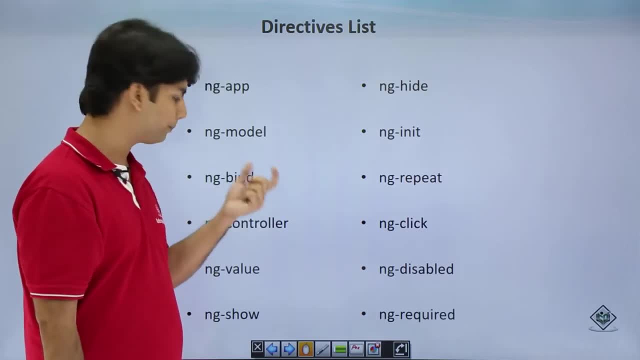 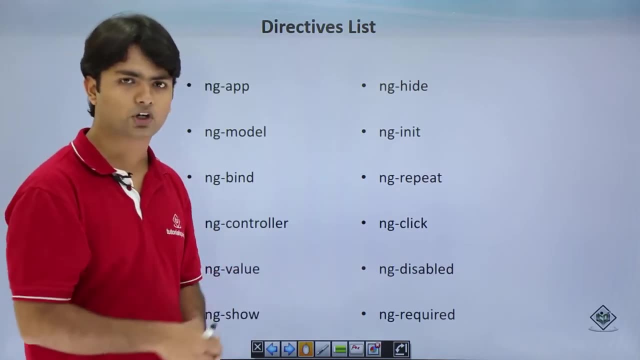 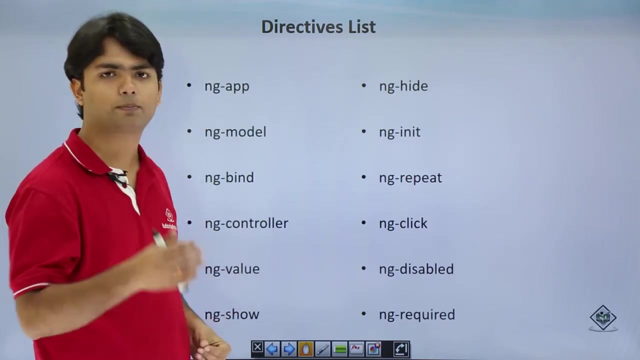 like span or any particular tag, use ng-bind, ng-controller, as I just discussed about it. whenever you want to specify which controller I am going to use on a particular segment, you can go for ng-controller, ng-value if you want to bind a particular value with any. 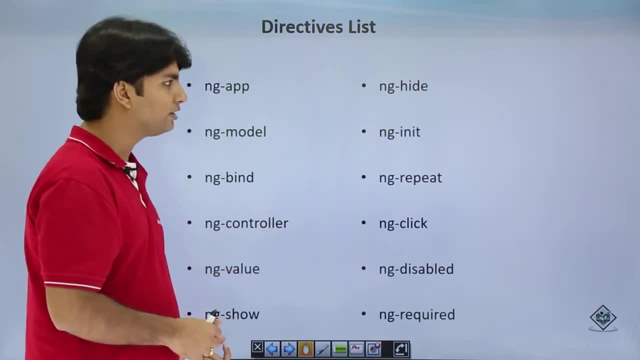 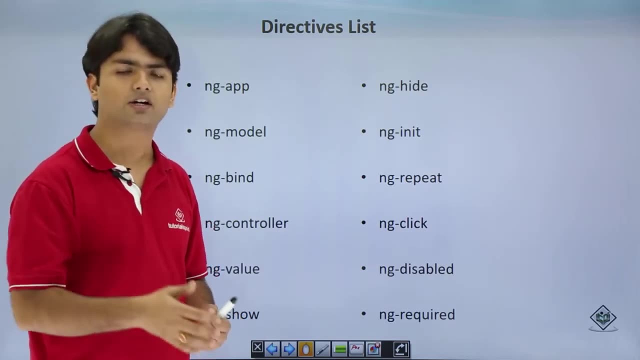 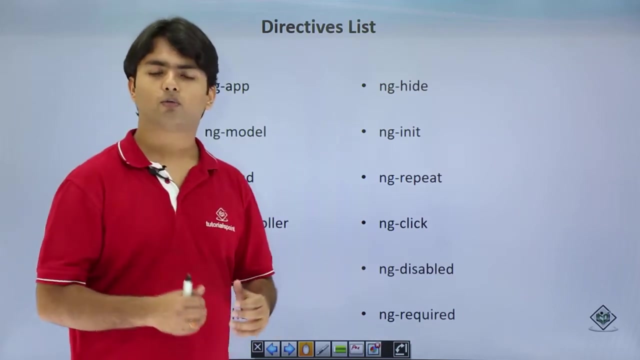 particular tag. in the sense Then ng-show, ng-hide. They are quite similar. as the name says. If programmatically you want to show or hide any control from the DOM, you can go for these two options. After that, ng-init, when you want to initialize any value with. 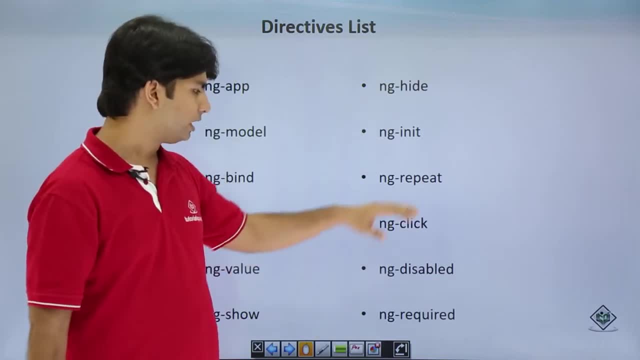 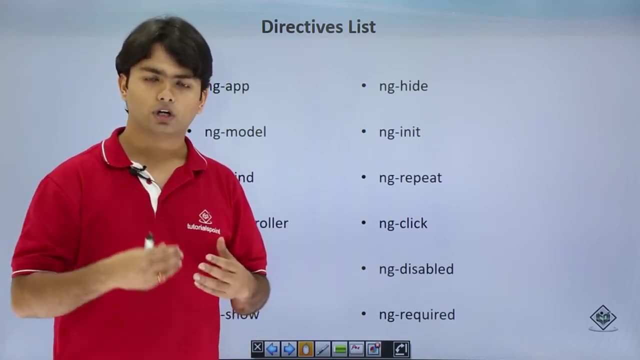 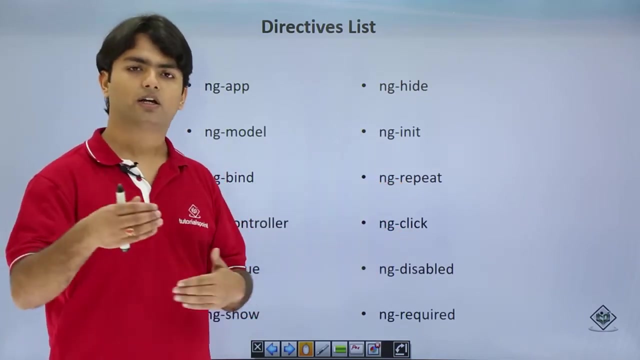 a particular value, any variable with a particular value, ng-repeat will be used as a loop. Suppose we have number of records and we want to put them inside the table, or any ordered, unordered list. So we can use ng-repeat so that it will execute so many times as the number of 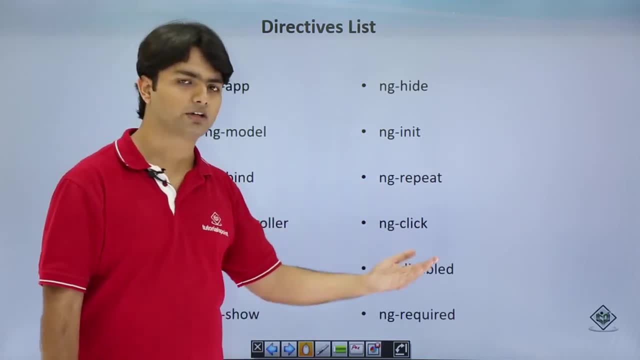 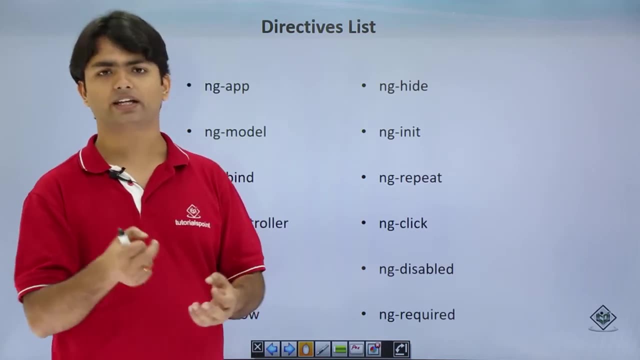 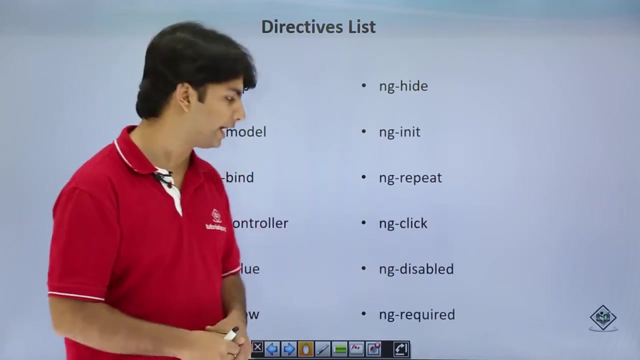 records we have. ng-delete or some relative directive will be used for the event-driven application. Suppose you want to make any function call or any action whenever you click a button or any particular event, So you will go for ng-click. at that time ng-disabled will be. 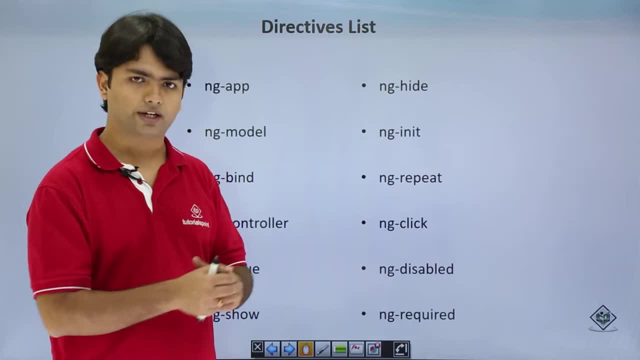 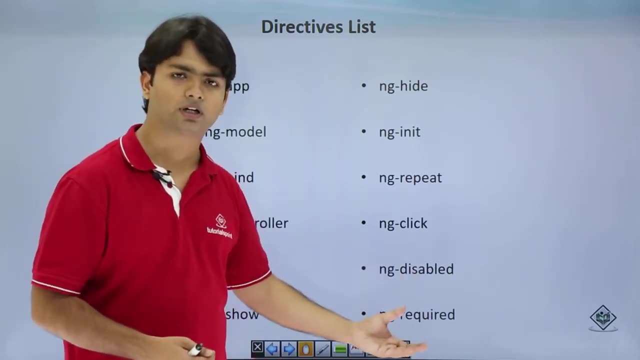 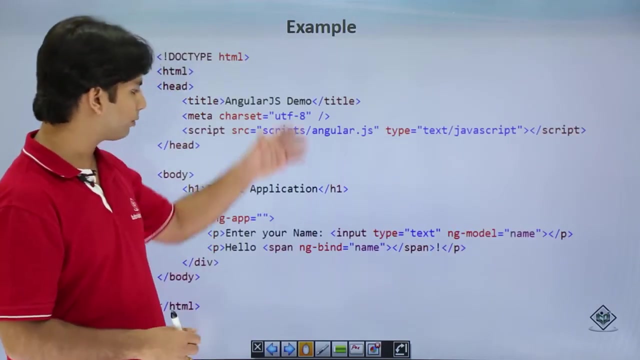 used to enable or disable the controls at the runtime And ng-required. suppose you want to make some form validations, you will get ng-required and some similar directives for putting the validations. So here we have a program in which we have implemented a couple of directives like ngModel and ngBind. 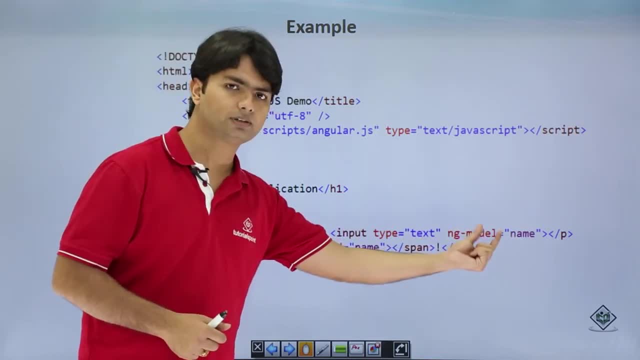 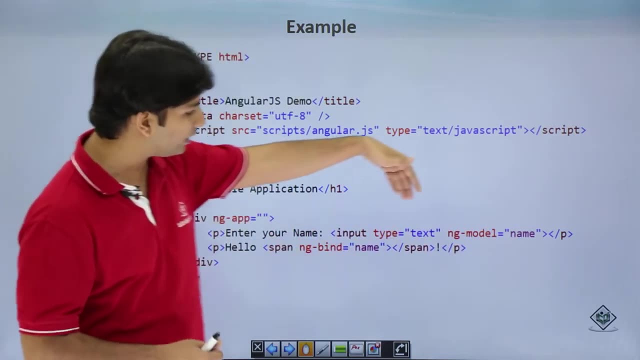 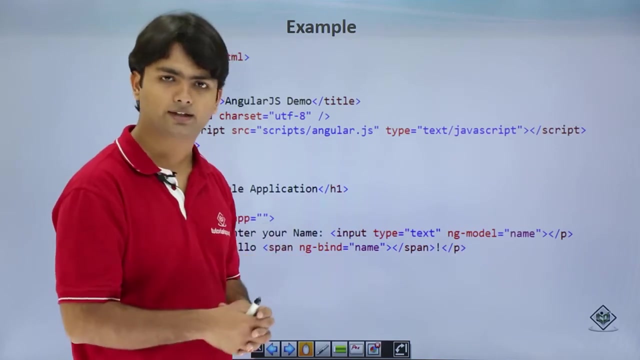 So, as I said that, when it is a control, I use ngModel with the value called name and the same value we have passed in span. So whatever you will enter in this text box will be shown here in this span. So let's see how this implementation will look like. 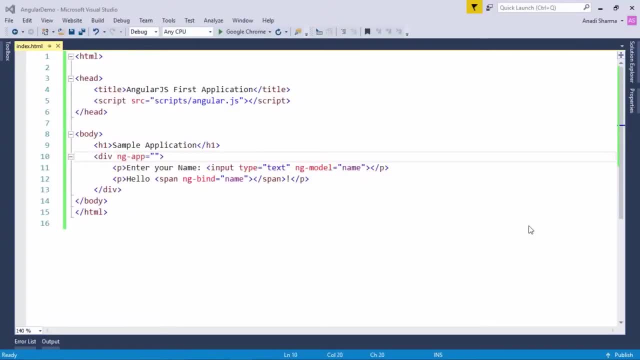 So now let's have a look how can we implement the directives in our AngularJS program. So, like the previous program, first of all I will have to include this Angularjs, which is here in my script folder. If you want, you can use the CDN path as well, directly from the AngularJS website. 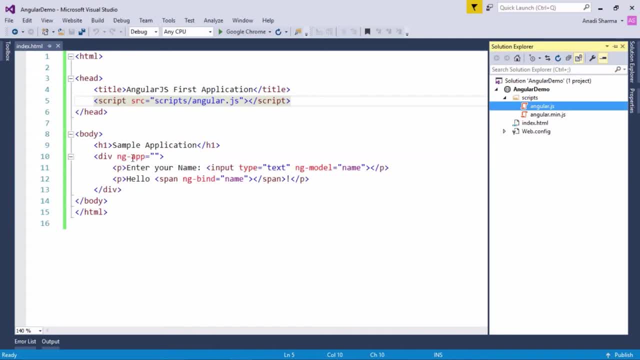 Now here, as we said that ngApp is the directive using which we can start the implementation of the directives. So let's say I want to take a text box of Angular in any HTML web page. Now, after this, I have taken a text box for taking the name of the user and I have used ngModel as the names, as the directive here. 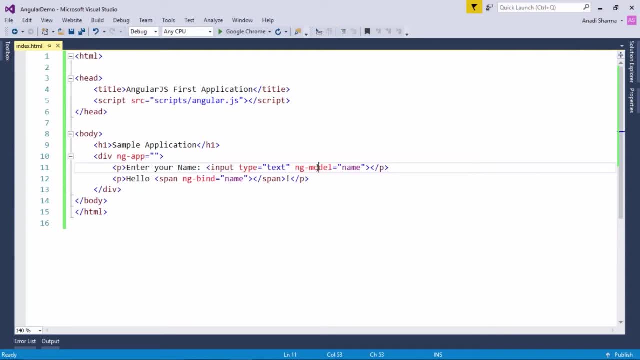 So this ngModel will actually bind the value with the HTML text box. that is a control. Now to the same thing with a tag like span is a tag out here. We will use the ngBind whenever I want to bind a value with a tag. 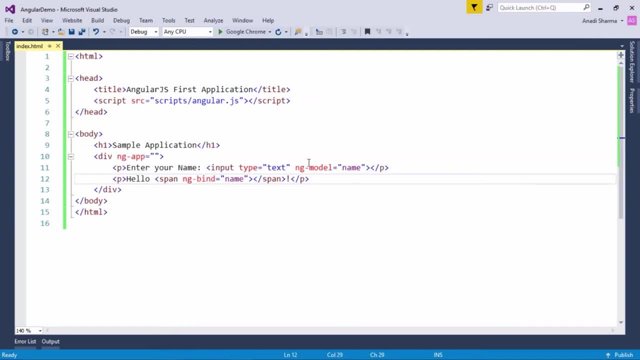 So, as I said, to bind it with a control, we will use ngModel, and to bind it with a tag, so we will use ngBind. So whatever we will start typing in this text box will get the same result here in the span as well. 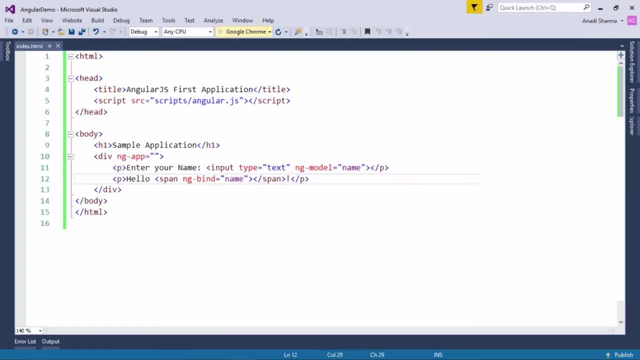 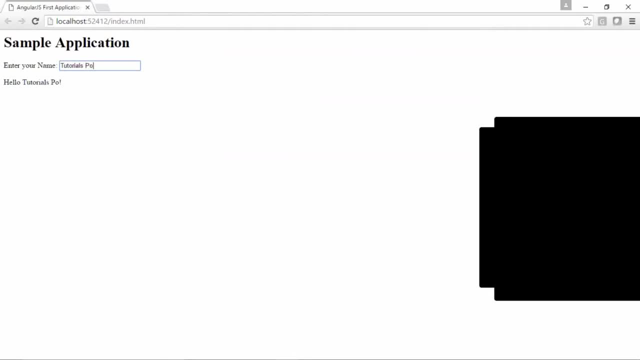 So let's see how the output will look like here. So here is the text box. I will start typing anything Right, So you can find. Whatever I entered here in this text box, the same I am getting here in the output. This is nothing but a span. 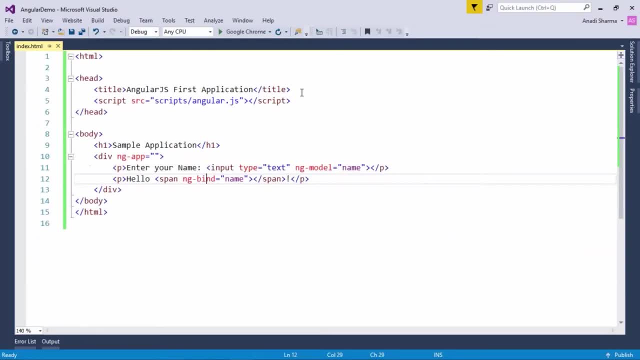 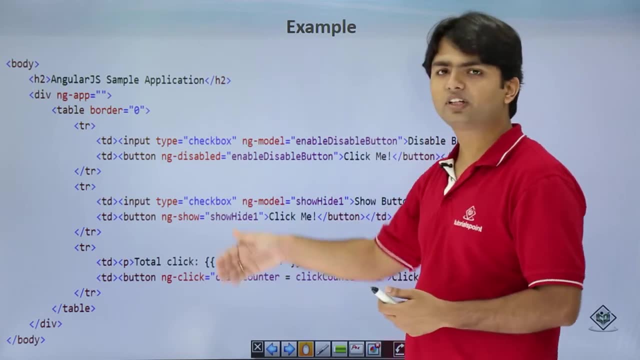 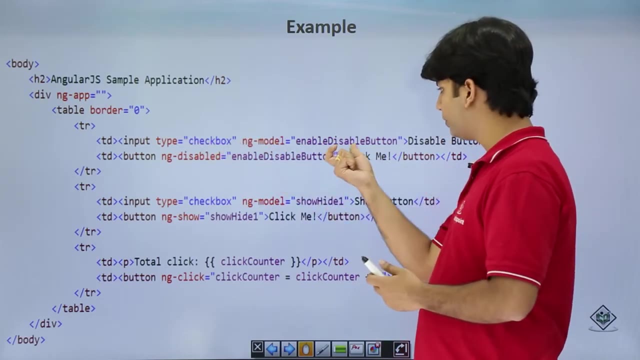 So this is how you can use the binding things in the AngularJS using ngModel and ngBind And similarly here you can see in another example we have used some more directives, Like here: in the first row you can see there is a checkbox with the ngModel enable- disable button. 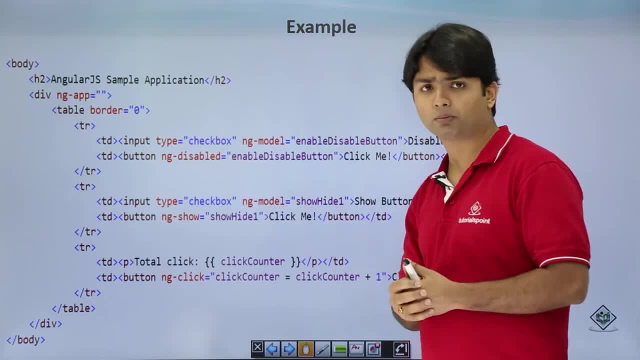 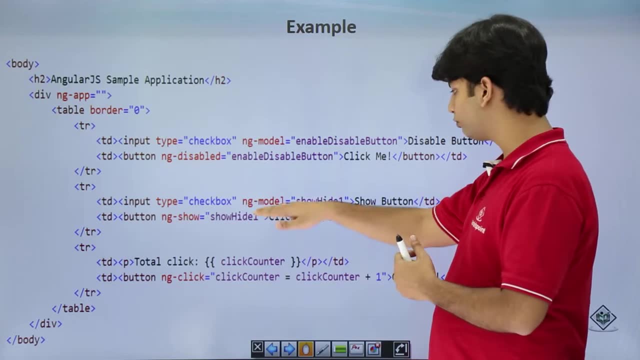 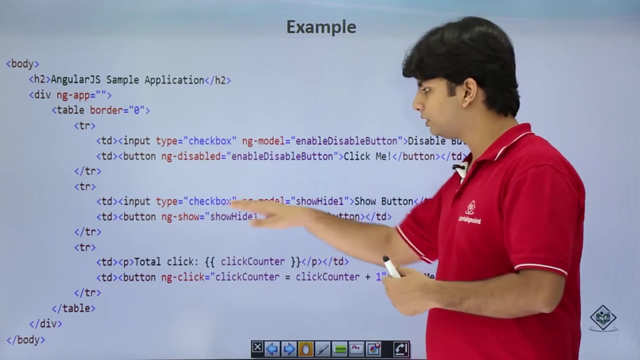 And here I have used the same name with the ngModel, So whenever you will check the checkbox, the button will be disabled. Similarly, in the second row we have used ngModel as showHide1 and used the same name with the ngShow. So whenever you will check the button, the button will be shown. 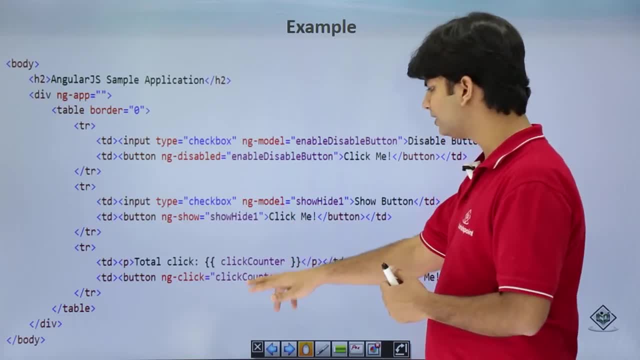 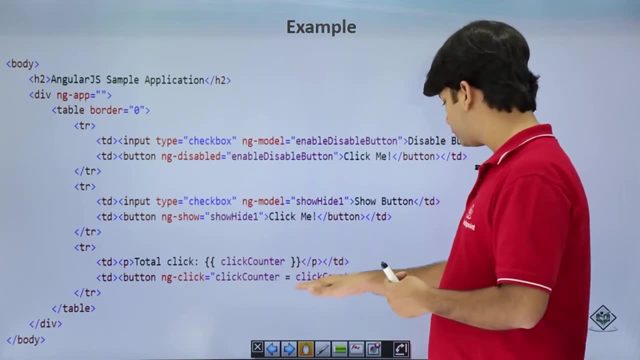 When you will uncheck it will be hidden. And here you can see there is a ngClick means I am using an event. So there is a variable called clickCounter which would be incremented every time with 1. Whenever you will click the button. 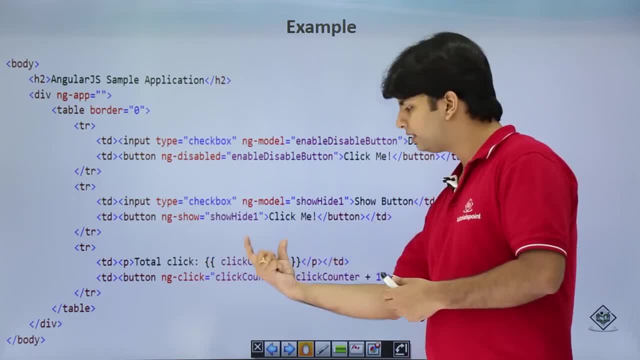 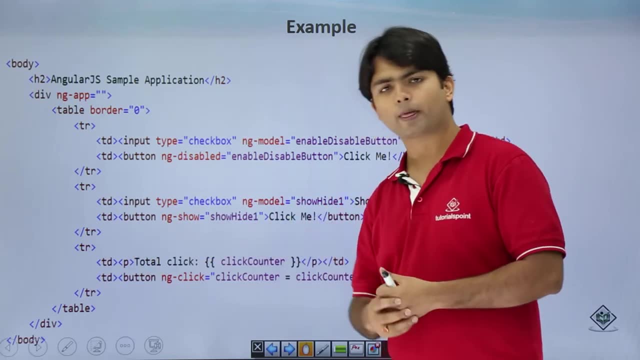 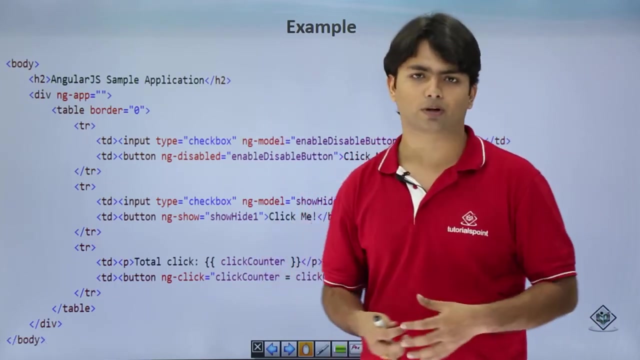 And you can see here I have printed the value in the expression Rather than using the expression. you can also go for ngBind for binding this particular value with the paragraph, Any way you want to put it. So let's see quickly how the implementation will look like. 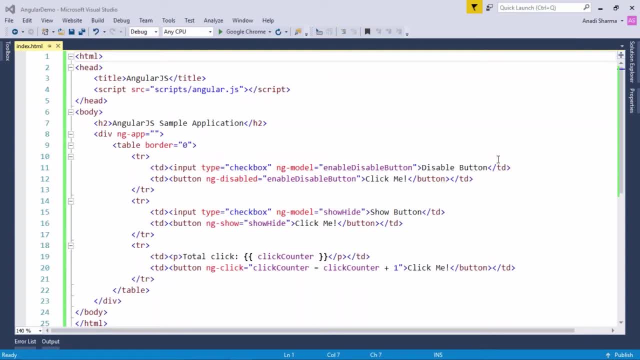 So here in the another example of directive you can find, like here in this table, I have taken 3 rows And in each row I have done a different operation. Like here, in the first row I have taken a checkbox with the ngModel named enableDisableButton. 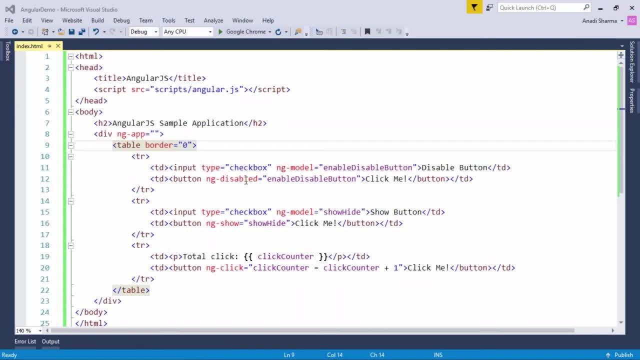 And right here, while working with the button, I have used ngDisableDirective, in which I am using the same name, that is, enableDisableButton. So as soon as you will check the checkbox out there, the model will become true, So as the disable will also be true. 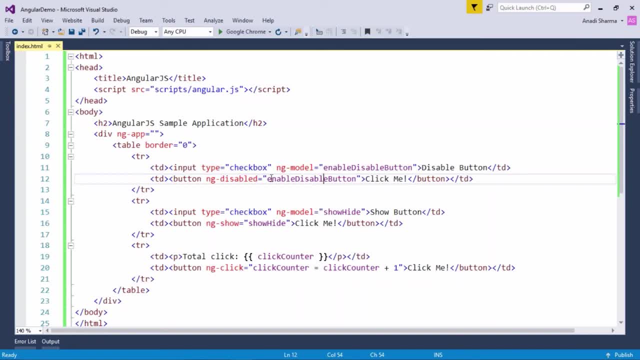 That simply means that when I will check the checkbox, the disabled will be true. So the button will get disabled, And when I will uncheck the checkbox, the button will be enabled again. So let's see whether it is doing the same or not. 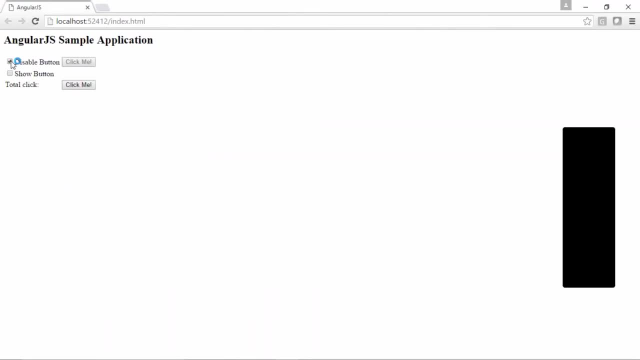 So you can see here: by default your checkbox is unchecked and the button is enabled as well. But as soon as I am clicking here on this checkbox, the button is disabled and no more clickable. So this is what we have done in the first row. 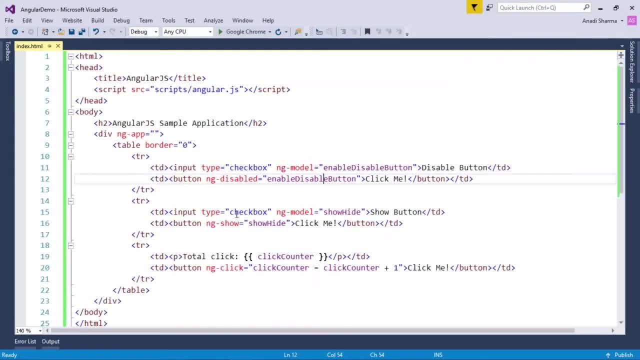 Let's find out what we have done in the second. Here in the second row, we have again taken a checkbox with the show hide model name and we have used ngShow. So whenever the checkbox is checked, the show will be true. So on the check of the checkbox, the button will be visible, and as soon as you will uncheck that, the button will be invisible again. 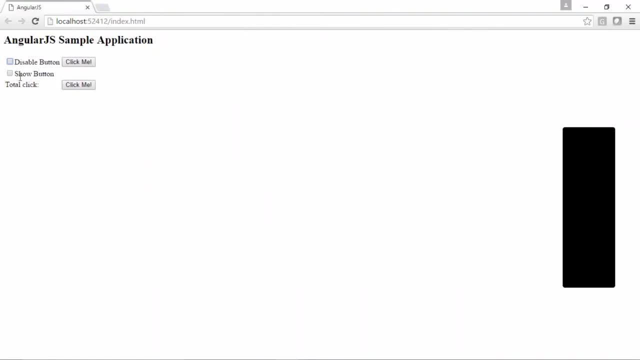 So let's see that. So here, as you can see, by default the checkbox is unchecked and you can't see any button right here. But as soon as I will check it, you can see. yes, there is a button. And as soon as I will do it again, the button is invisible. 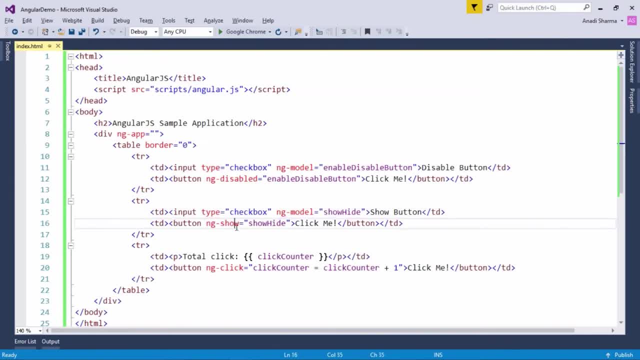 Right. So this is how the ngDisabled and ngShow buttons are working. Now in the third example, what we have taken is we are using the click event on AngularJS for a button. So in the ngClick directory, What we have done is we are just incrementing the click counter variable by one. 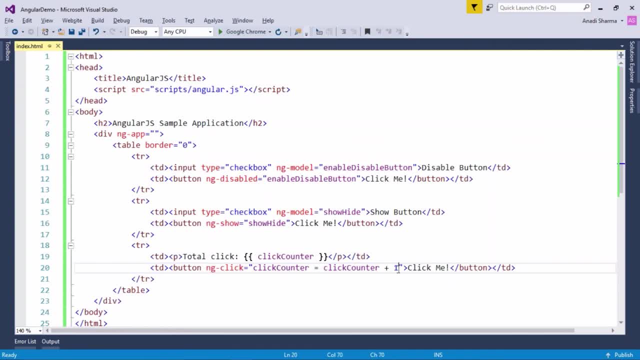 By default, it would be initialized with the zero. Whenever you will increment it with one, you can see that particular value to be printed right here in this first td, As we know that we can also use the ngBind directive to bind any particular value with the HTML tag.